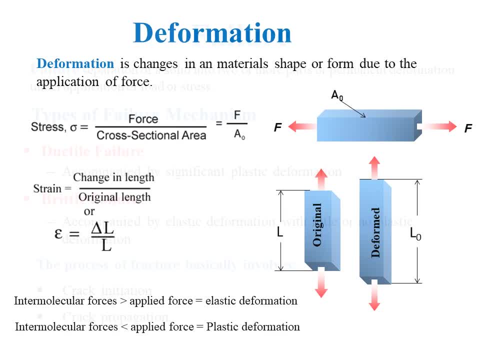 and elastic deformation. As we know, when force or stress is applied on a plastic material, its shape changes. This change in shape is known as deformation. During deformation, the intermolecular forces of the material oppose the applied force. If the intermolecular force 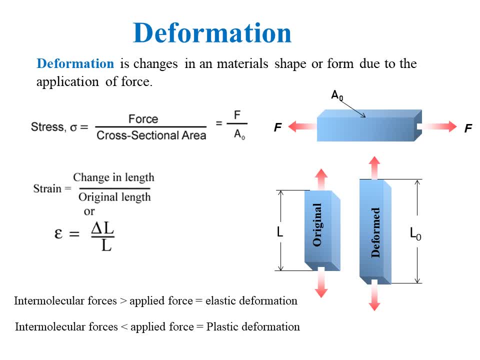 is large enough to resist applied force, the samples returns to its original state when load is removed. This is known as elastic deformation. If the intermolecular force is not sufficient enough to overcome the force, then it is called elastic deformation applied force. then the sample undergo permanent deformation. It cannot go back. 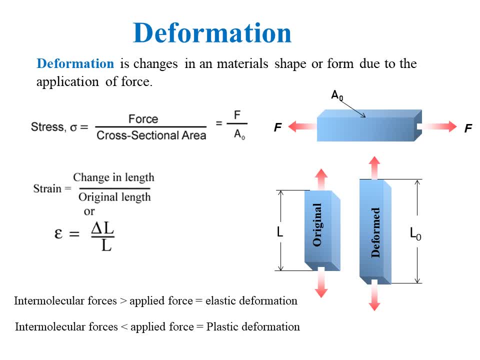 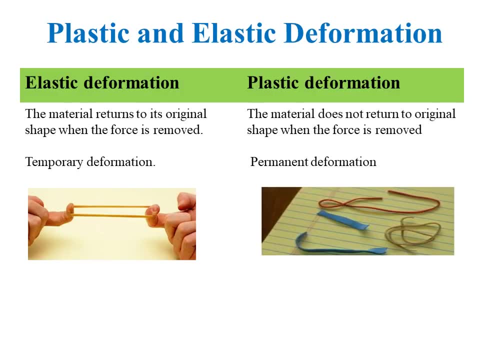 to its original shape even after the force is removed. This type of deformation is known as plastic deformation. At microscopic level, elastic deformation occurs in the form of bond stretching and rotation, which is temporary. The best example for elastic deformation comes from elastomers such as elastic rubber. When we pull the elastic rubber band on the ends it. 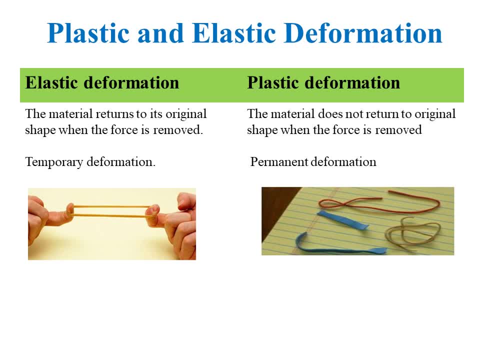 stretches. If we stop pulling it, it comes back to its original shape. This shows phenomena of elastic deformation. but when pulling force is very high and it breaks the material shows plastic deformation. Plastic deformation is permanent and irreversible deformation. It occurs due to breakage of limited 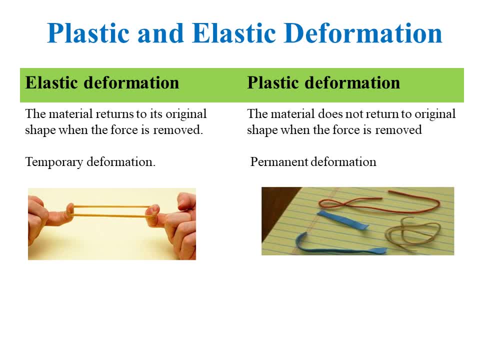 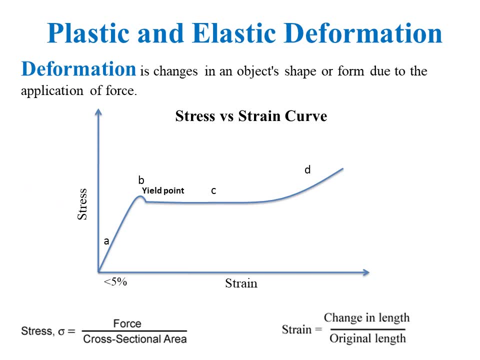 number of chemical bonds. If we look at stress-strain curve of a polymeric material, we can see that amount of stress required to deform a polymeric material changes with extent of deformation, As elastic deformation occurs at very low strain value, which is less than five percent, and plastic deformation occurs at relatively. 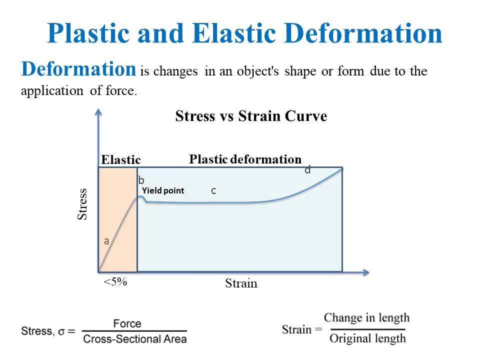 high strain value. In elastic region, stress increases linearly with strain, which indicates materials resistance to deformation. At certain point, which is known as yield point, materials resistance to deformation decreases As a result. material can be easily deformed. In this phase we can see that strain. 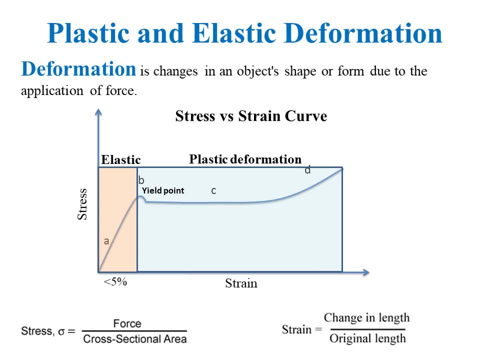 increases without increase in stress indicating stretching or elongation in material. The yield point is the point that indicates the limit of elastic behavior and the beginning of plastic behavior. So those plastic materials that fail at very low strain are known as brittle material, and those who requires high energy to break or fail at high strain are known as. 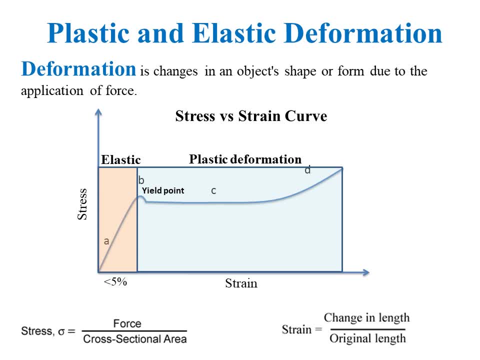 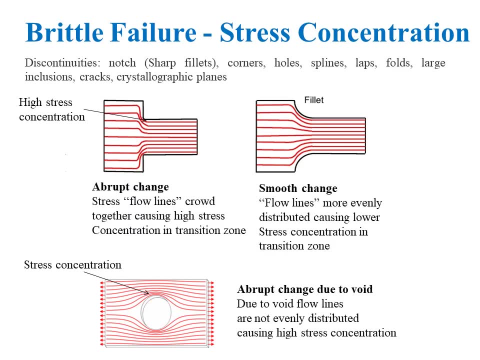 ductile material. The mechanism by which brittle and ductile material fail is know as brittle-material limitation. For localbility, theеруplasticference is required to be more appropriate device in your��th undergo. Know alpurg6 and ductile failure. The main cause of brittle failure is stress concentration. 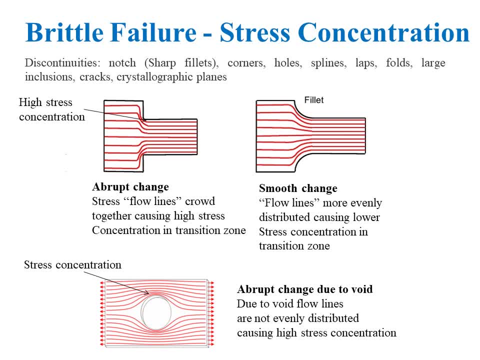 that is present in the structure of molded or manufactured product. Discontinuities that develop during molding or service life initiate crack formation. The discontinuities can be in the form of notch corners, holes, splints, flaps, folds, large inclusions, cracks, crystallographic planes, etc. 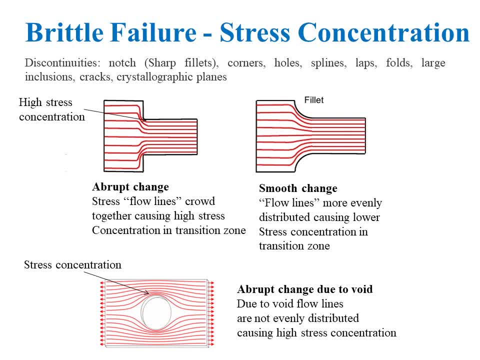 A stress concentration, which is also known as a stress razor, is a location in an object where stress is concentrated. An object is stronger when force is evenly distributed over its area, So a reduction in area, for example, caused by crack or void, results in localized increase in. 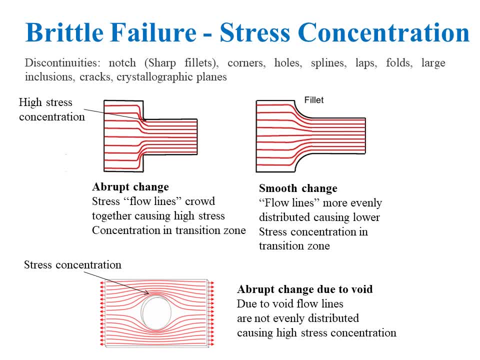 stress, So stress concentration- is an area in a material or a sample where force is not evenly distributed and force accumulates there. When force in that area become larger than what the material is supposed to withstand or designed to withstand, it starts to crack, As we can see here. in case of sample having a void, the line of force are not 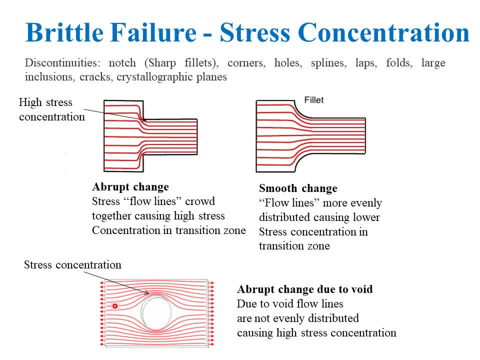 straight near the void, as the line of force has high density near the void compared to rest of the area. therefore material starts to crack from here. Brittle failure is worst type of failure because the surface is the being. it involves the sudden failure of the material by rapid crack growth immediately after the 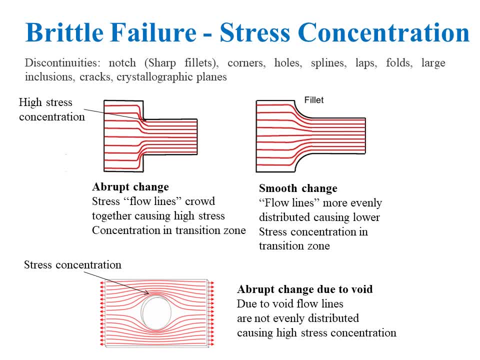 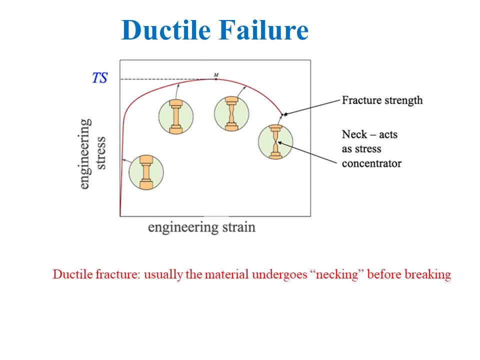 crack initiation. This type of failure is also known as fast failure. A classic example of ductile failure is tensile specimen. Ductile failure provides some warning. before failing. The material deform, elongates and decrease in cross section before failure. Elongation and decrease in cross section refers to necking. That means usually the material undergo. 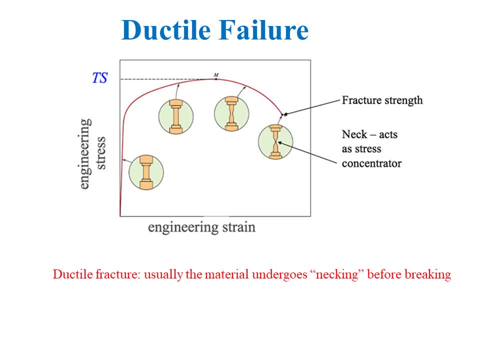 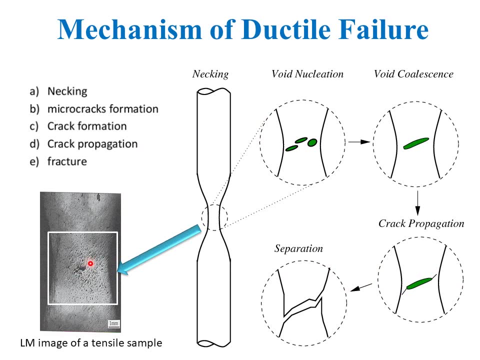 necking before breaking, Whereas brittle failure is quick and no prior warning, This sample starts to fracture due to the formation of the micrvoids in the neck region. These microvoids grow in size and begin to join together or totemy. 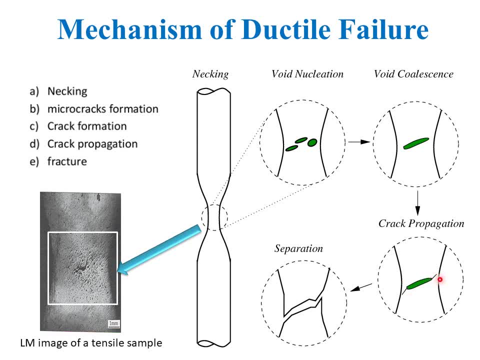 to produce an internal crack. The final separation of the cross section occurs by shear rupture. In ductile failure there is absorption of massive amount of energy. therefore crack propagation occurs very slowly before the fracture. That is why plastic deformation occurs at a very high strain value, because material undergo large deformation before failing. 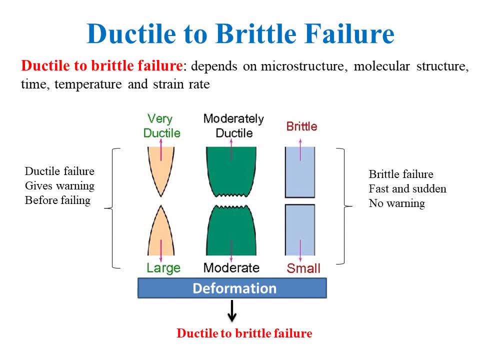 So we learn about two extreme behaviors of a material, which are brittle and ductile failures. But many of the polymeric materials fails in ductile to brittle manner. That means many polymeric conditions can make a plastic partially ductile and partially brittle. Therefore, most of the plastics show intermediate ductility, unless they are deliberately made. 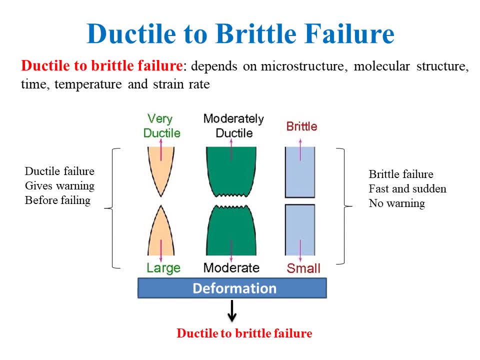 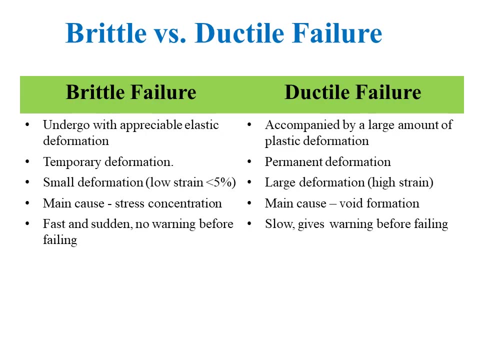 to be very ductile or very brittle. This ductile to brittle transition depends on microstructure, molecular structure, time, temperature and percentage strain. In summary, we can say that brittle failure undergo with appreciable elastic deformation and high ductility, And ductile failure occurs with plastic deformation. Elastic deformation is reversible and temporary.